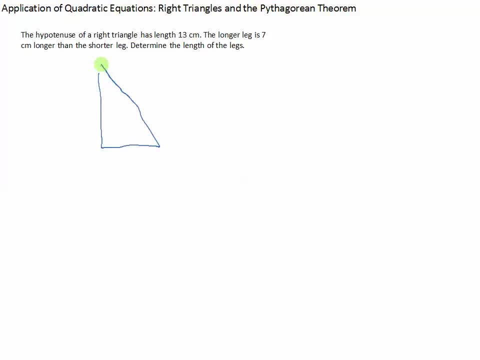 So let's draw a right triangle here And start labeling things. We know the hypotenuse is 13 centimeters. The longer leg, So we'll of course assume that's the vertical leg, is 7 centimeters longer than the shorter leg. 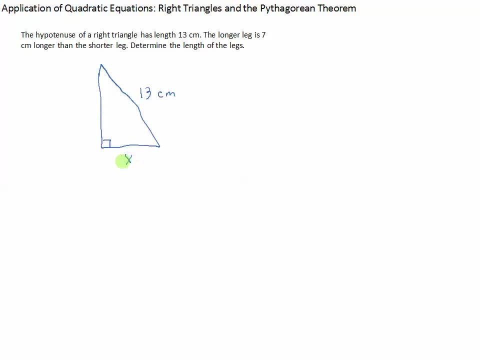 So let's call the shorter leg x, So x represents the length of the short leg. Then the long leg has to be that short leg plus 7, because it's 7 more than the shorter leg. So now our Pythagorean Theorem tells us that if I take this leg squared, 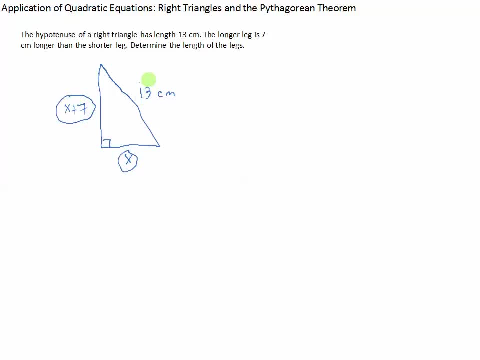 plus this leg squared, I get 13 squared. So let's set that up. We end up with x squared plus x plus 7 squared equals 13 squared, And lo and behold, we get a quadratic equation. Let's get rid of all these parentheses. 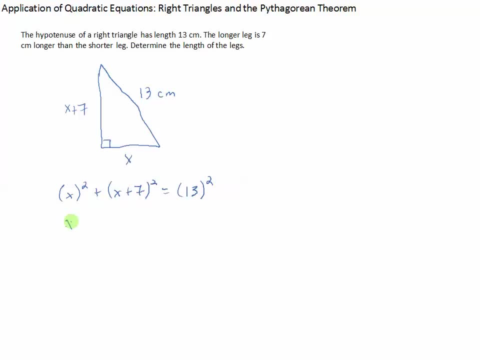 so that we can see what we're dealing with. x squared is easy. That's just x squared. You don't need the parentheses there. x plus 7 squared, though, is x plus 7 times x plus 7.. Be very careful in doing this. 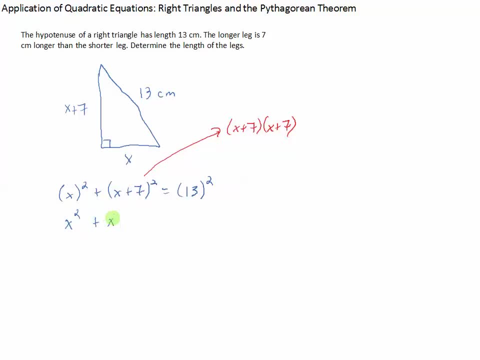 So if you were to multiply all this out, you would get x squared plus 14x plus 49 equals 13 squared, which is 169.. Now maybe we'll combine all our terms and get 0 on one side. So x squared plus x squared is 2x squared plus 14x. 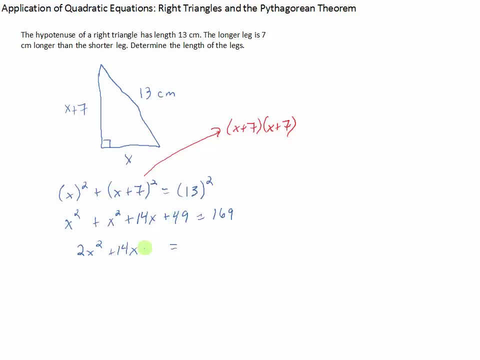 And then if I subtract 169 from 49, I get negative 120 equals 0.. And now solve this quadratic equation using whatever technique you like. This one in particular factors, so you can try that. It's a trinomial. 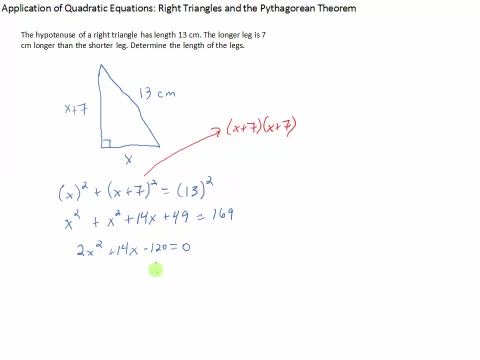 Factor the 2 out first, of course, But when you do, you should end up with x equals negative 12 or x equals 5.. Well, x represents the length of the short leg, So there's no possible way that x could be negative 12..